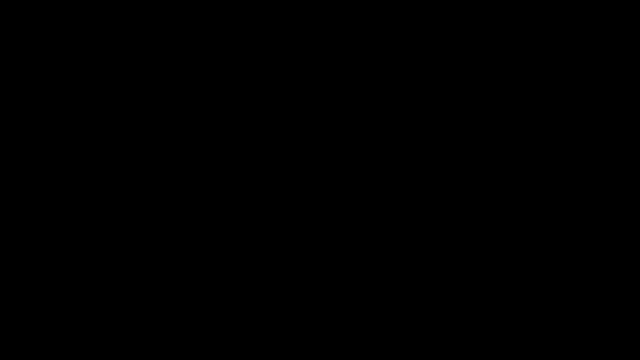 In this video, we're going to focus on integrating exponential functions, So let's go ahead and begin. What is the antiderivative of e to the x dx? What do you think the answer is For this function? it's simply going to equal the same thing. It's e to the x plus c. 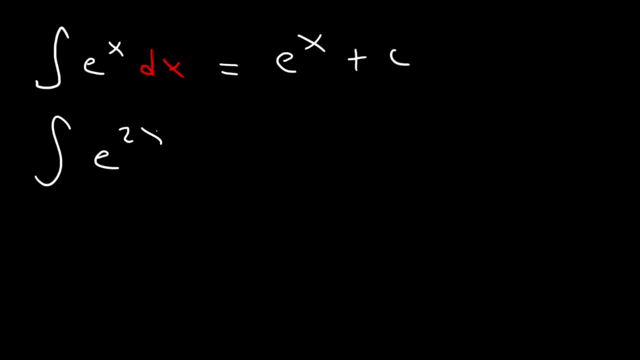 Now, what about this one? What is the antiderivative of e to the 2x dx? This is going to be e to the 2x divided by the derivative of 2x, which is 2, plus c. That technique works only if you divide it by a constant. 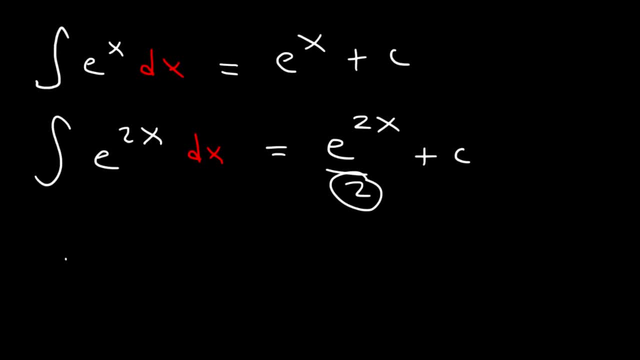 If you divide it by a variable, it's not going to work. So what do you think? the answer for this one is e to the negative 5x, dx. It turns out that It's going to be the same thing: e to the negative 5x divided by the derivative of negative 5x, which is negative 5, plus c. 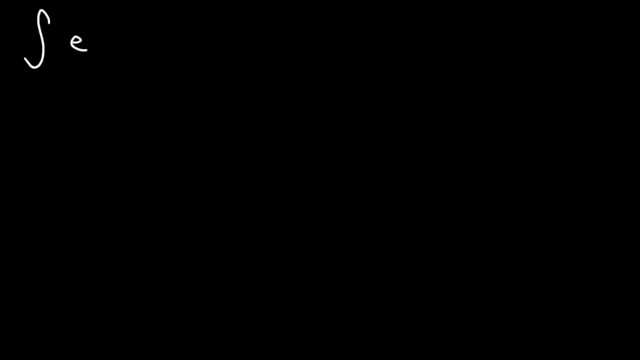 Now let's prove the last one using u substitution. So let's make u equal to negative 5x. du is the derivative of negative 5x, which is negative, 5.. times dx and solving for dx, it's du divided by negative 5x. 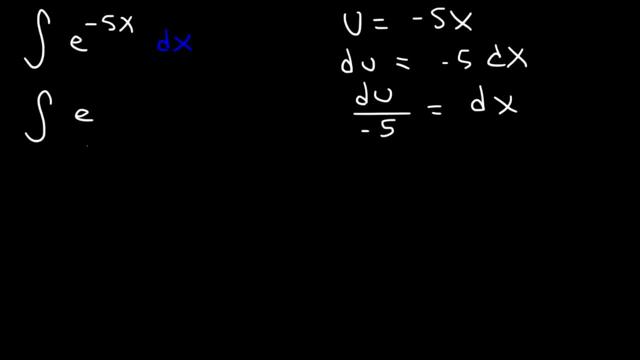 so now let's replace negative 5x with the u variable and let's replace the dx with du over negative 5. now let's take the constant negative 5 and let's uh move it to the front so it's negative 5, antiderivative of eu or e to the u du. 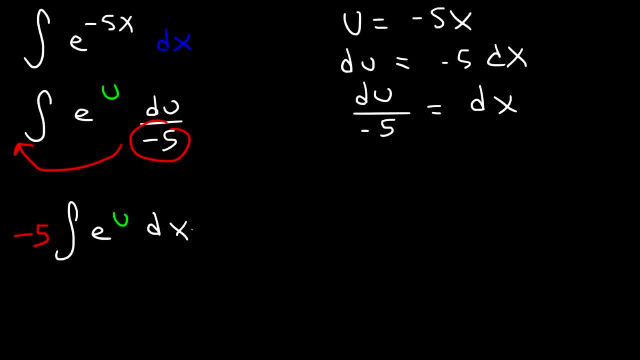 now we know that the integration of each x is simply each dx. so the antiderivative of e to the u is simply e to the u plus c. and now we can replace u with negative 5x. so the final answer- oh, by the way, this should be negative 1 over 5, because the five is on the bottom- 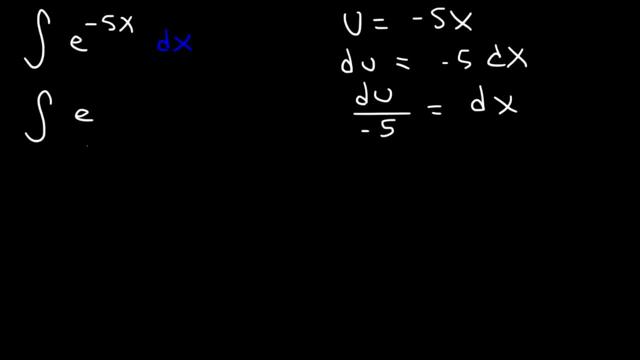 so now let's replace negative 5x with the u variable and let's replace the dx with du over negative 5. now let's take the constant negative 5 and let's uh move it to the front so it's negative 5, anti-derivative of eu or e, to the u du. 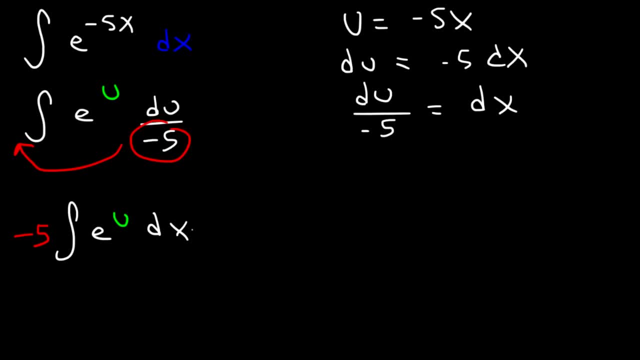 now we know that the integration of e to the x is simply e to the x, so the anti-derivative of e to the u is simply e to the u plus c. and now we can replace u with negative 5x. so the final answer- oh, by the way, this should be negative one over five, because 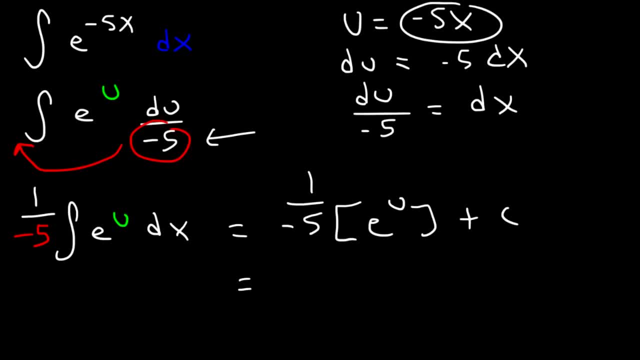 the five is on the bottom, so just keep that in mind. i almost forgot about that, but the final answer is negative one over five e to the negative five x plus c, which is the same thing we just did: negative one over five e to the negative five x plus c. 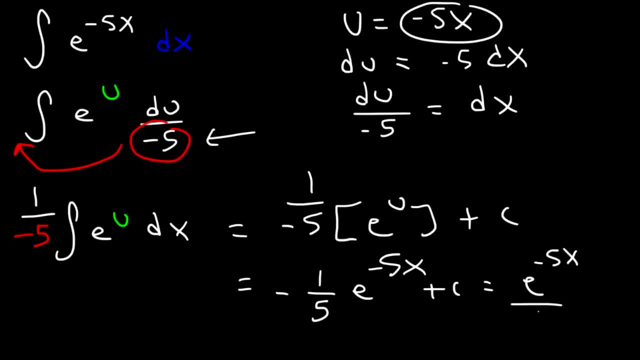 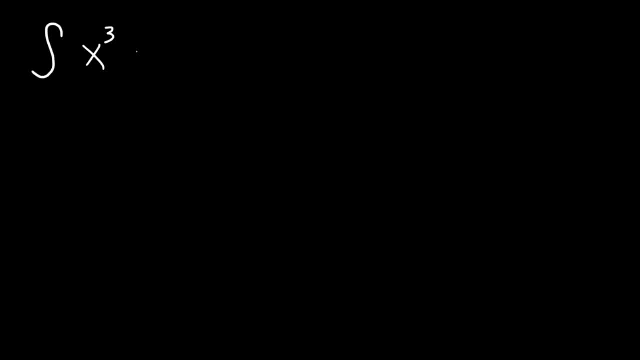 thing as what we have, which was e to negative 5x divided by negative 5 plus c. Here's another one: x cubed times e raised to the x to the fourth, dx. Go ahead and integrate the function, So we can integrate by substitution. Let's replace u with x to the fourth, So therefore. 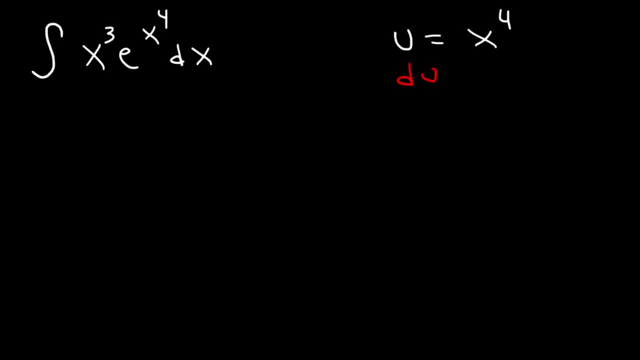 du is going to be the derivative of x to the fourth, which is 4x cubed times dx. And now let's solve for dx, That's du over 4x cubed. So let's replace x to the fourth with the u variable. 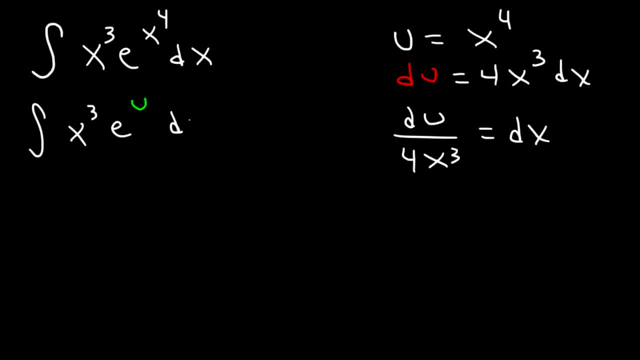 And now let's replace dx with du over 4x cubed, And so we could cancel x cubed. Now let's move the 4 to the fourth, So it's 1. fourth anti-derivative e to the u du. The integration of e to the? u is just: 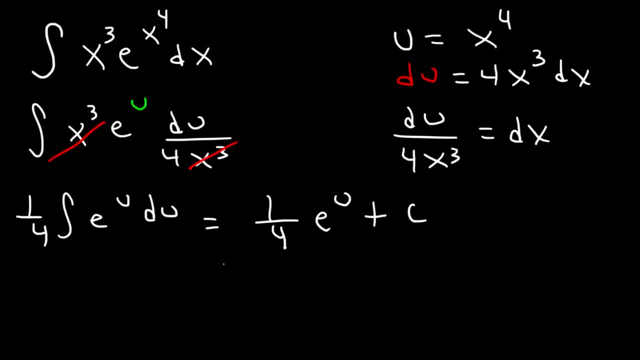 e to the u times 1 fourth plus c, And now all we need to do is replace u with x to the fourth. So the final answer is 1 fourth e raised to the x to the fourth plus c, And, as you can see, it's not that bad. So that's it for that problem, And now let's move on. 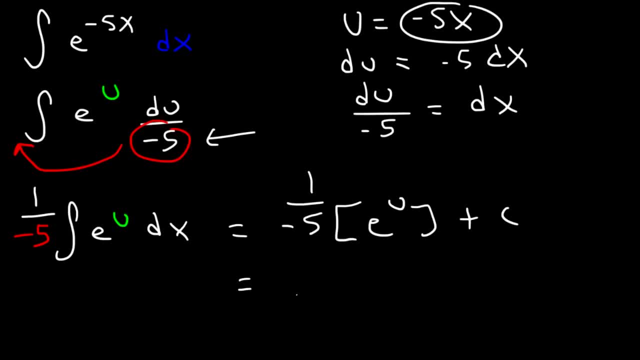 so just keep that in mind. almost forgot about that. but the final answer is negative 1 over 5, e to the negative, 5x plus c, which is the same thing as what we have, which was e to negative 5x divided by negative 5 plus C. Here's another one: x cubed times e raised to the x to the. 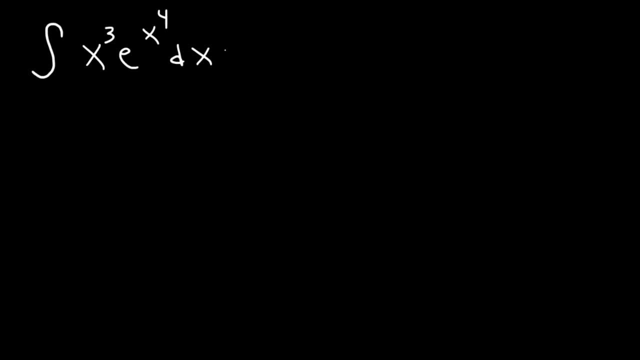 fourth dx. Go ahead and integrate the function. So we can integrate by substitution. Let's replace u with x to the fourth. So therefore, du is going to be the derivative of x to the fourth, which is 4x cubed times dx. and now let's. 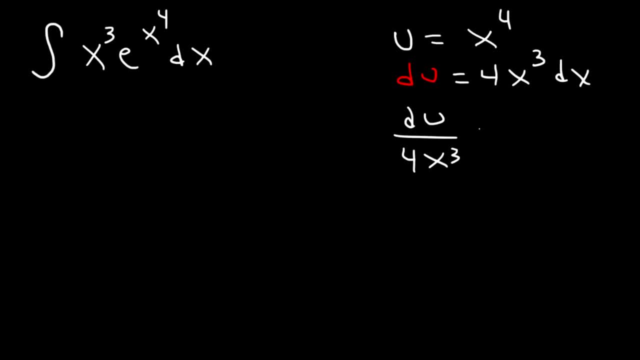 solve for dx, That's du over 4x cubed. Let's replace x to the fourth with the u variable and now let's replace dx with du over 4x cubed. We could cancel x cubed. Now let's move the 4 to the front, So it's 1 fourth. 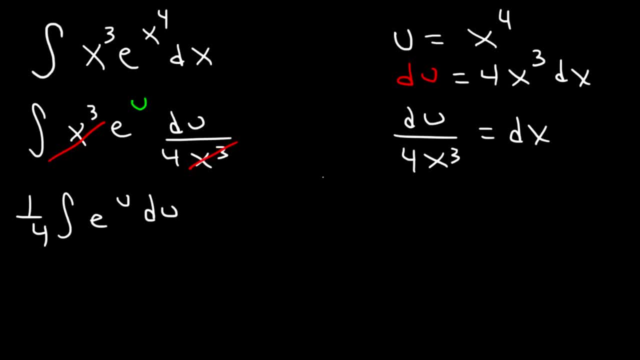 antiderivative e to the u du. the integration of e to the u is just e to the u times one-fourth plus c, and now all we need to do is replace u with x to the fourth. so the final answer is one-fourth e raised to the x to the fourth plus c, and, as you can see, it's not that bad. so that's it for. 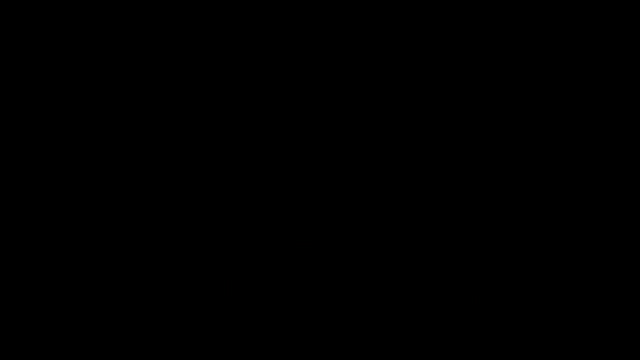 that problem. and now let's move on to the next one. here's another one. you could try: e to the x times the square root of one, minus e to the x, dx. so what do you think we need to do first? in this example, we should make u equal to one, minus e to the x. if we do that, 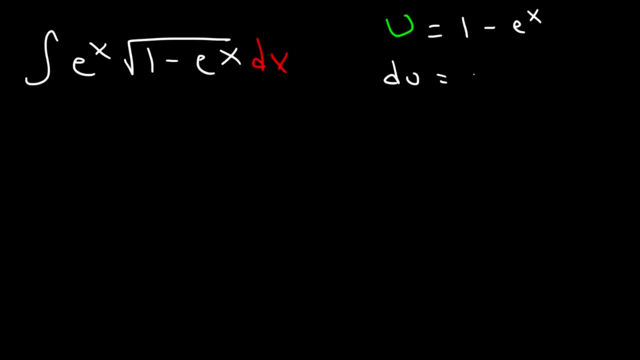 du is going to be negative e to the x. dx. the derivative of one is zero. the derivative of e to the x is e to the x, so the derivative of negative e to the x is negative e to the x. now, solving for dx, it's du over negative e to the x, so this is going to be e to the x times the square root of u. 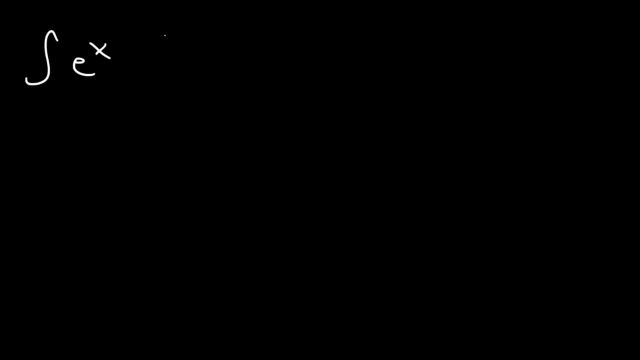 to the next one. Here's another one you could try: e to the x times the square root of 1 minus e to the x dx. So what do you think we need to do first? in this example, We should make u equal to. 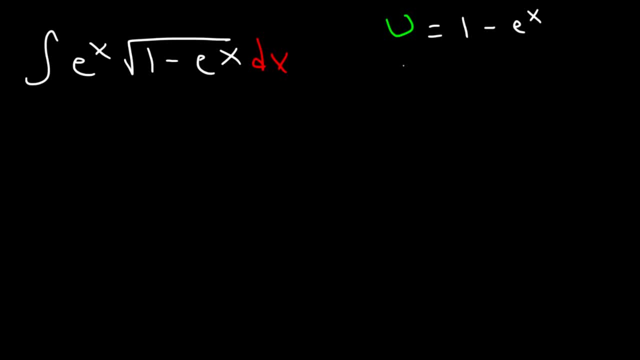 1 minus e to the x. If we do that, du is going to be negative e to the x, dx. The derivative of 1 is 0.. The derivative of e to the x is e to the x. So the derivative of negative e to the x. 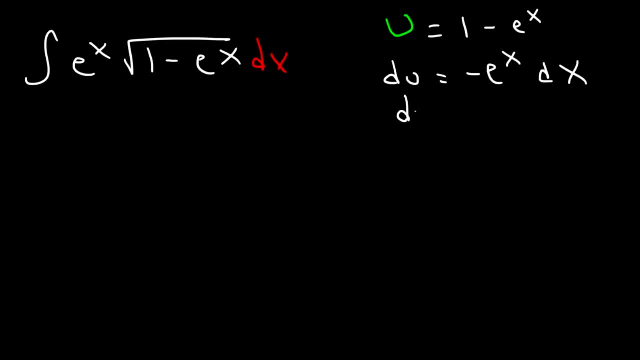 is negative e to the x. Now solve for dx. It's du over negative e to the x, So this is going to be e to the x times the square root of u and dx is du divided by negative e to the x. So we can: 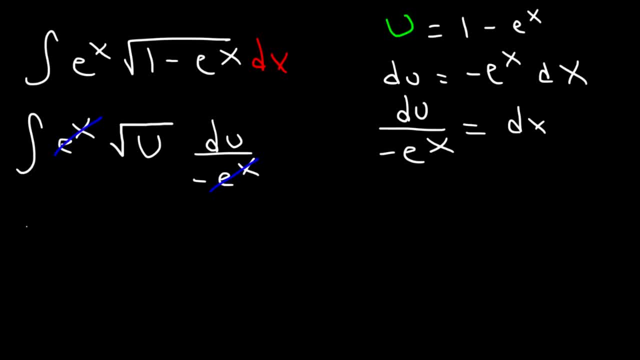 cancel e to the x So we can move the negative in front. the square root of u is basically u to the one half and then times du. So now let's integrate, let's add one to the exponent. one half plus one is three over. 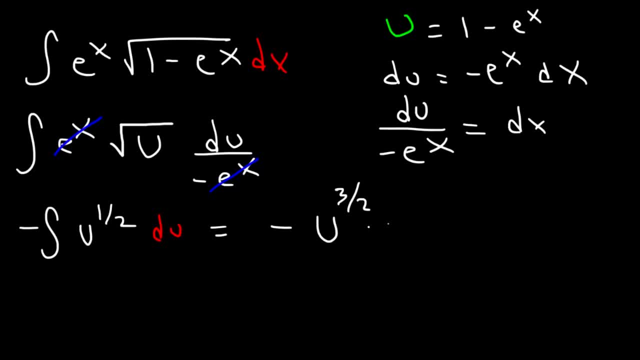 two, and instead of dividing it by three over two, we can multiply it by two over three. Let's add the constant c. So now we need to replace u with one minus e to the x. So the final answer is negative: two over three, one minus e to the x, raised to the three over. 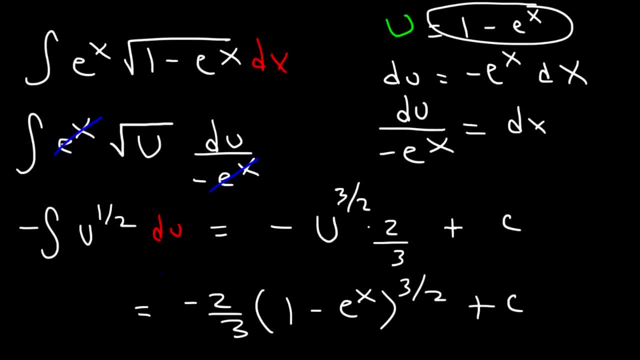 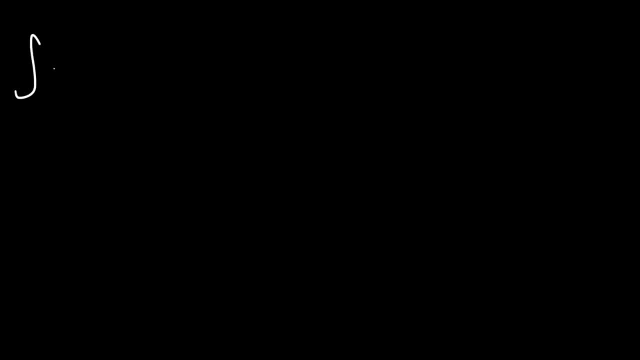 two plus c, And that's it for this problem. Here's the next one: e to the x plus, e to the negative, x divided by e to the x minus, e to the negative, x, dx. So listen carefully, Let's integrate this. 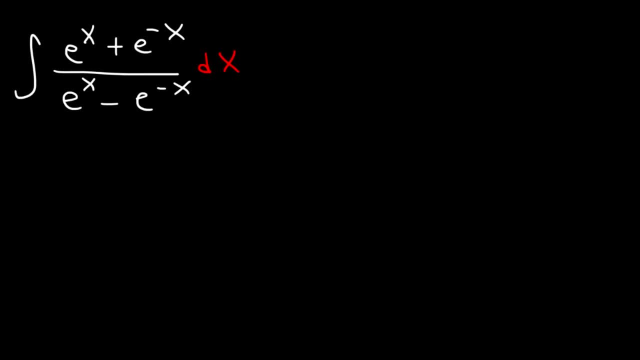 What should we make u equal to The bottom one or the top one In this problem? we want to make u equal to the bottom one so we can get rid of the top one. So u is going to be e to the x minus e to the negative x. 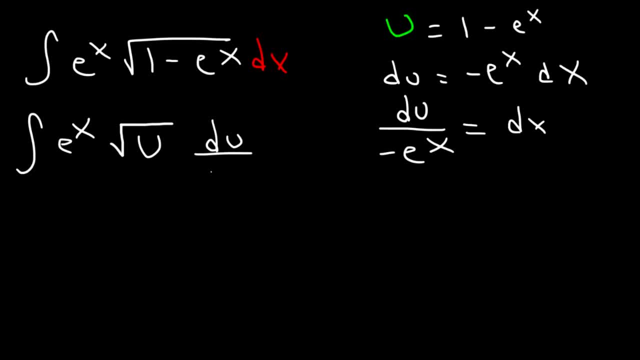 and dx is du divided by negative, e to the x, so we can cancel e to the x, so we can move the negative in front. the square root of u is basically u to the one half and then times du. so now let's integrate, let's add one to the exponent. one half plus one is three over two, and instead of dividing, 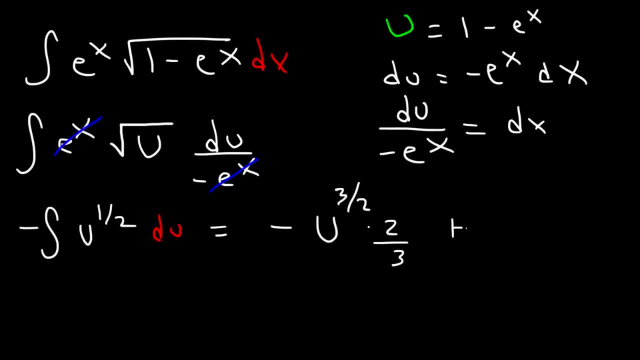 it by three over two. we can multiply it by two over three. let's add the constant c. so now we need to replace u with one minus e to the x. so the final answer is negative: two over three, one minus e to the x and raised to the three over two plus c, and that's it for this problem. 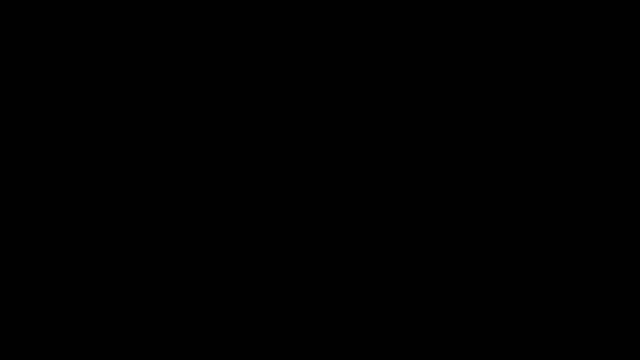 here's the next one: e to the x plus, e to the negative, x divided by e to the x minus, e to the negative, x, dx. so let's integrate this. what should we make? u equal to the bottom one or the top one in this problem? we want to make u equal to the bottom one, so we can. we can get rid of the top one. 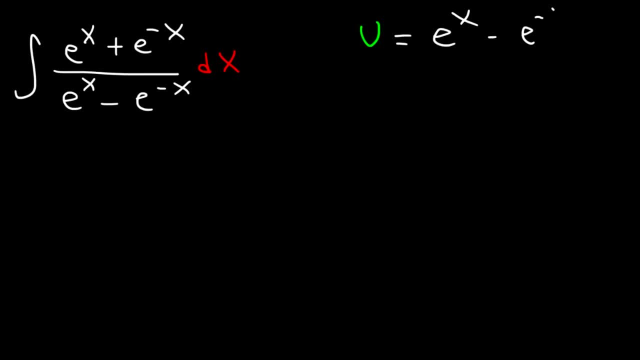 so u is going to be e to the x minus e to the negative x. so now let's find du. the derivative of e to the x is just e to the x. the derivative of negative e to the negative x is going to be negative e to the negative x times negative one, and all of this is multiplied by dx. 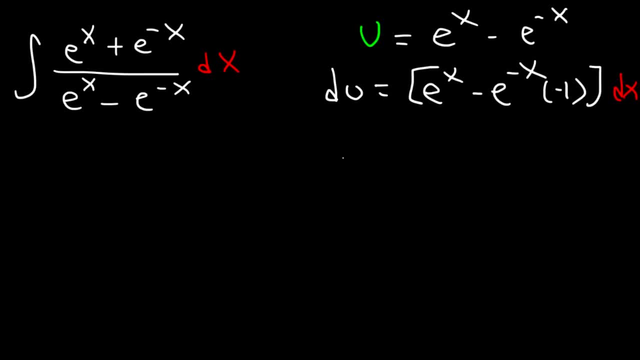 so negative e to the x times negative one is basically positive e to the negative x. so solving for dx it's du over e to the x plus e to the negative x, and this is good because we can see that this is the same as a numerator, which means that's going to cancel soon. so let's rewrite what. 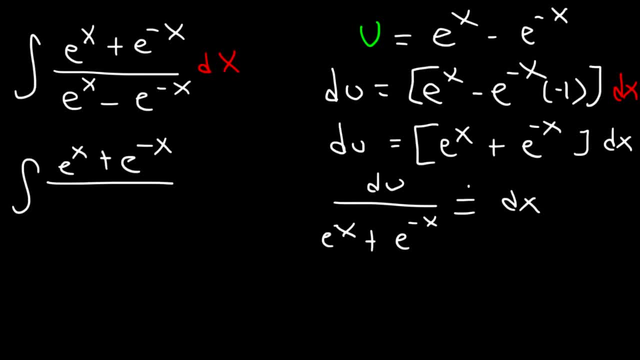 we have. let's replace the denominator with the u variable, because they're equal to each other, and let's replace dx with du over ex, plus e to the negative x, and so these two will cancel, and now what we have is the antiderivative of one over u du. 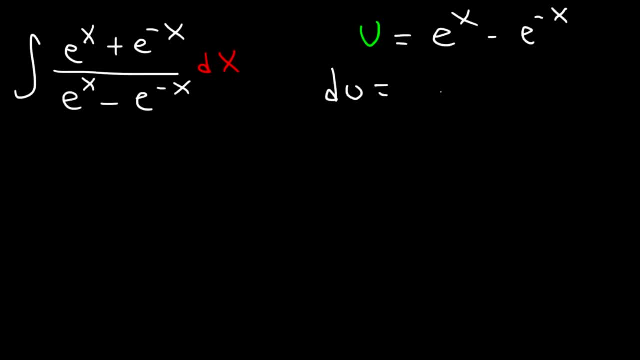 So now let's find du, The derivative of e to the x is just e to the x. The derivative of negative e to the negative x is going to be negative e to the negative x times negative one, And all of this is multiplied by e to the x. 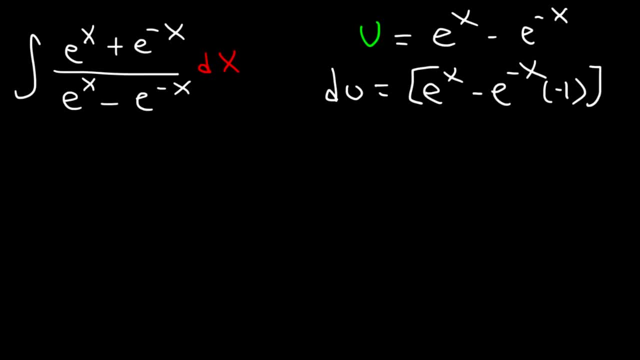 The derivative of negative e to the x is multiplied by dx, So negative e to the x times negative one is basically positive e to the negative x. So solving for dx it's du over e to the x plus e to the negative x. 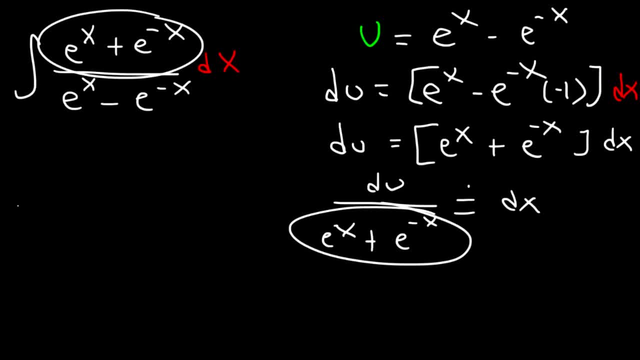 And this is good, because we can see that this is the same as the numerator, which means that's going to cancel soon. So we're going to have the derivative of e to the x plus e to the negative x. So let's rewrite what we have. Let's replace the denominator with the u variable, because they're equal to each other, And let's replace dx with du over ex plus e to the negative x, And so these two will cancel. 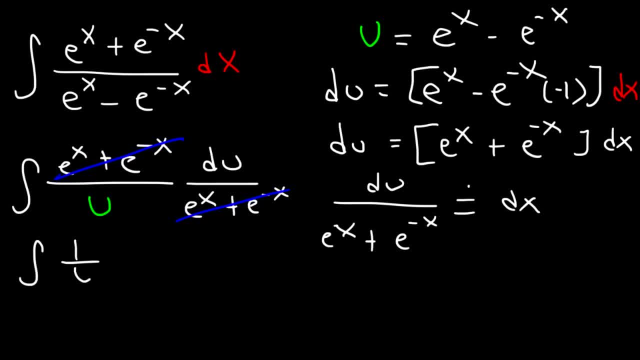 And now what we have is the antiderivative of 1 over u du, which is going to be ln u plus c, And now we can replace u with this. So the answer is the natural log of ecx minus e to the negative x plus c. 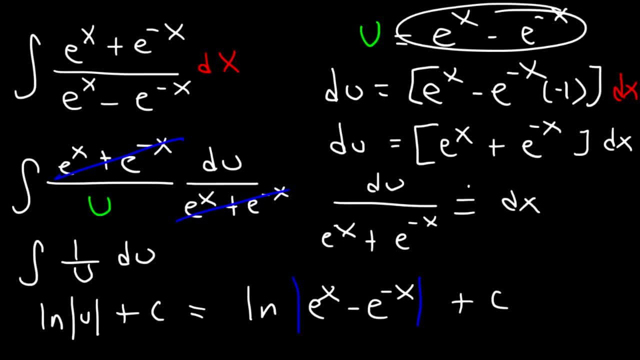 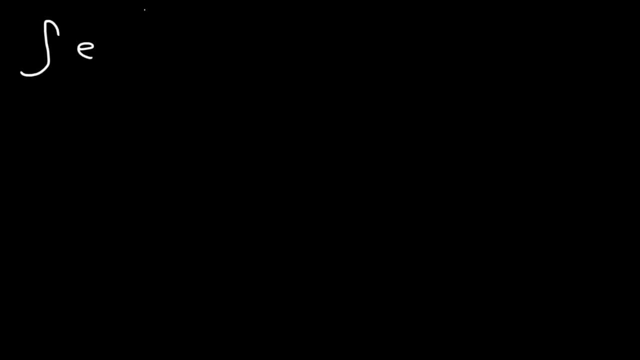 And let's put this in absolute value. And so this is the solution. Let's work on another one. e to the 1 over x squared divided by x cubed dx. So what do you think we should make u equal to In this example? let's make u equal to 1 over x squared. 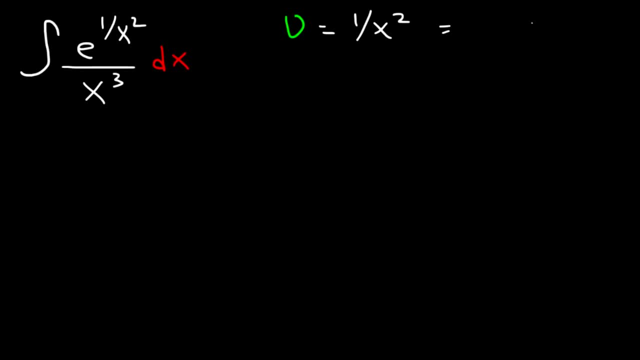 And before we find a derivative, let's rewrite it. This is equal to x raised to the minus 2.. So, du, using a power rule is going to be negative, 2x to the negative, 2 minus 1 or negative. 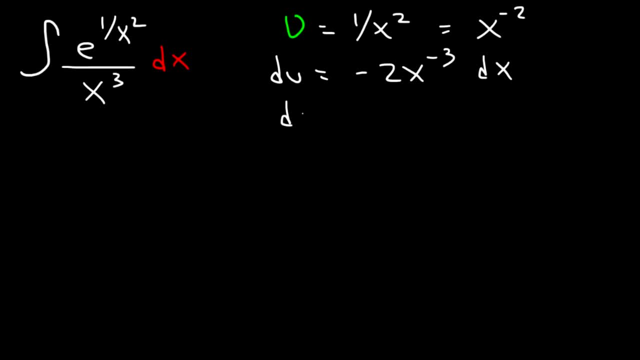 So du is going to be negative 3 times dx. Now, before we solve for dx, let's simplify, Let's get rid of the negative exponent. We can do that by moving x from the top to the bottom, So negative 3 will now become positive 3.. 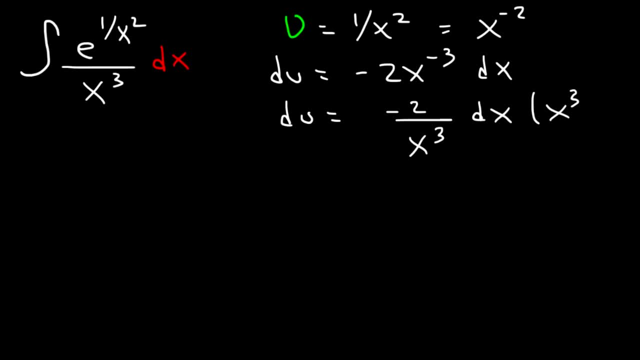 And now let's get dx by itself. So first let's multiply both sides by x cubed, So these will cancel. And so we have x cubed. du is equal to negative 2 dx. So now let's divide both sides by negative 2 to get dx by itself. 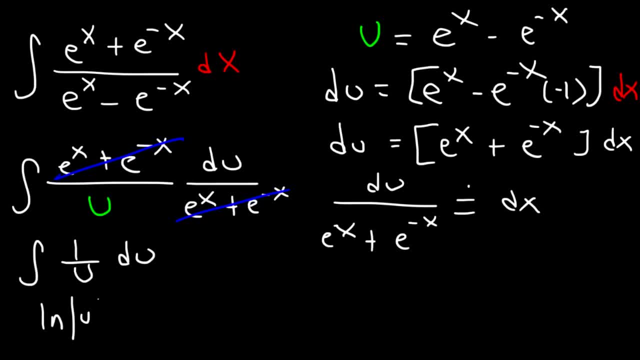 which is going to be ln u plus c, and now we can replace u with this. so the answer is the natural log of e to the x minus e to the negative x plus e to the negative x. so now we have negative x plus c, and let's put this in absolute value, and so this is the solution. 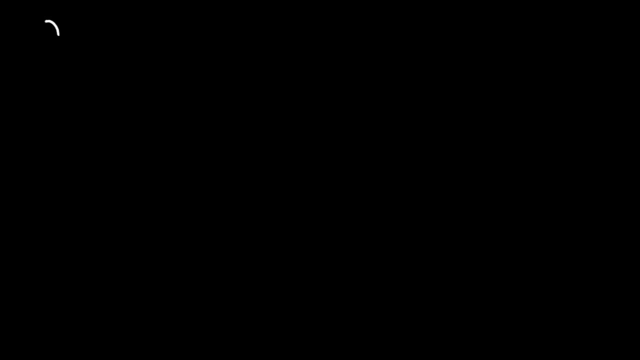 let's work on another one: e to the 1 over x squared, divided by x cubed dx. so what do you think we should make u equal to? in this example, let's make u equal to 1 over x squared, and before we find a derivative, let's rewrite it. this is equal to x raised to the minus 2, so, du. 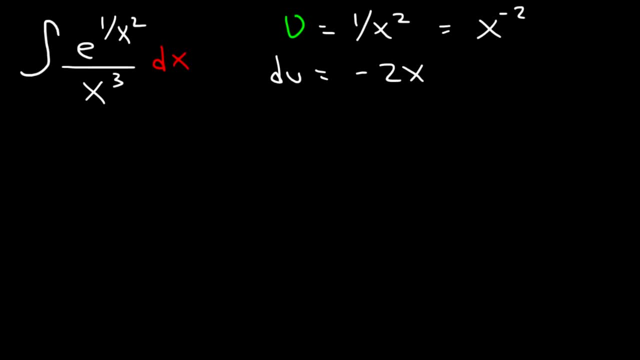 using a power rule is going to be negative 2, x to the negative, 2 minus 1, or negative 3 times dx. now, before we solve for dx, let's simplify. let's get rid of the negative exponent. we could do that by moving x from the top to the bottom, so negative 3 will now become positive 3. and now let's get. 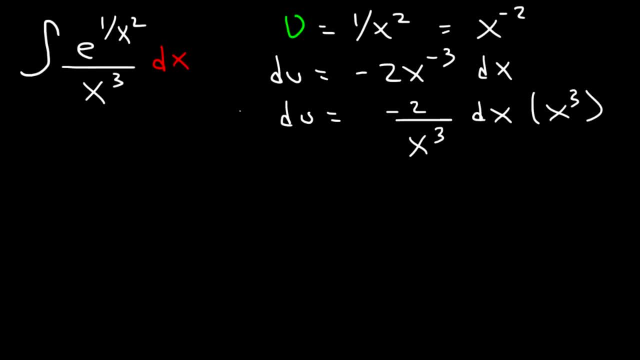 dx by itself. so first let's multiply both sides by x cubed, so these will cancel, and so we have x cubed du is equal to negative 2 dx. so now let's divide both sides by negative 2 to get dx by itself. so dx is equal to x cubed du divided by. 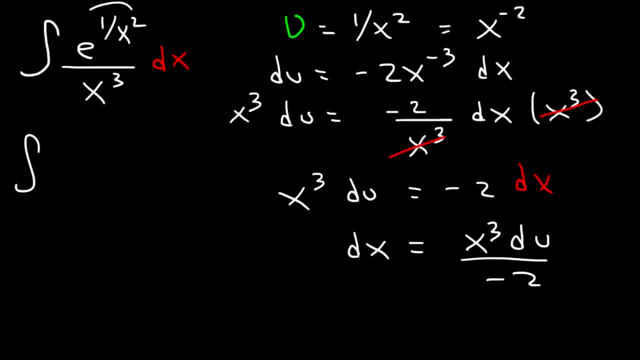 negative 2. so now let's replace 1 over x squared with u, so this is e raised to the u divided by x cubed, and let's replace dx with what we have here, and that's x cubed, du over negative 2. and so let's cancel x cubed and let's take the negative 2 move to the front. so it's going to. 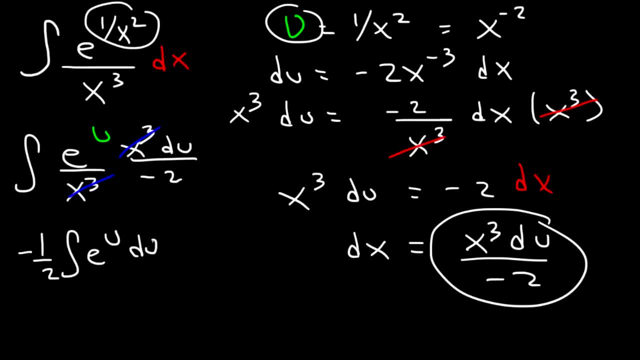 come out as negative one half integration e to the u du, which is equal to x cubed du divided by x cubed du. and so we have: x cubed du divided by x cubed is equal to negative 1 half e to the u plus c. and now all we need to do is replace u with what it. 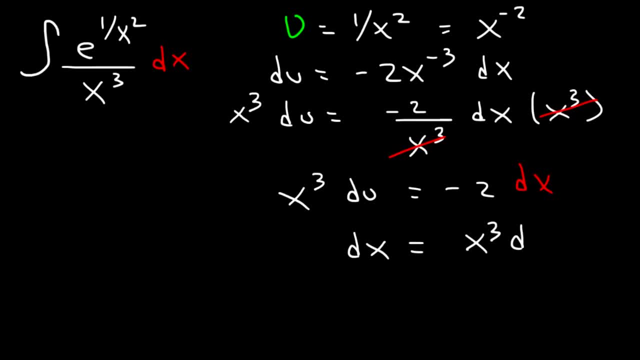 So dx is equal to x cubed du divided by negative 2.. So now let's replace 1 over x squared with u, So this is e raised to the u divided by x cubed, And let's replace dx with what we have here. 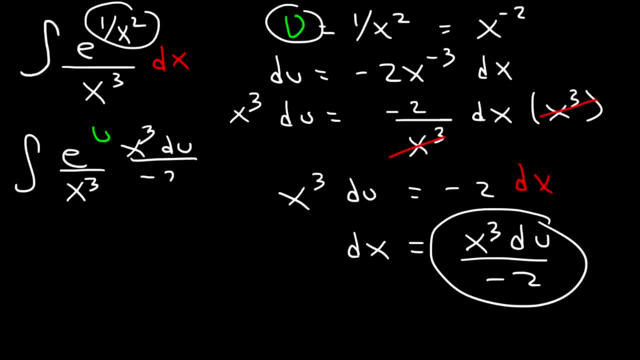 And that's x cubed du over negative 2.. And so let's cancel x cubed And let's take the negative 2 and move it to the front, So it's going to come out as negative 1 half integration e to the u du. 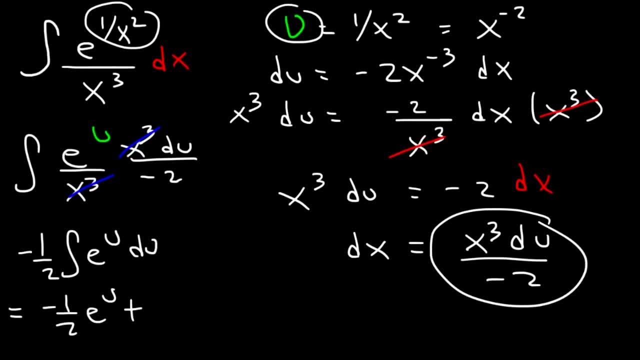 Which is equal to negative 1 half e to the u plus c. And now all we need to do is replace u with what it was. So the answer is going to be negative 1 half e to the 1 over x squared plus c. 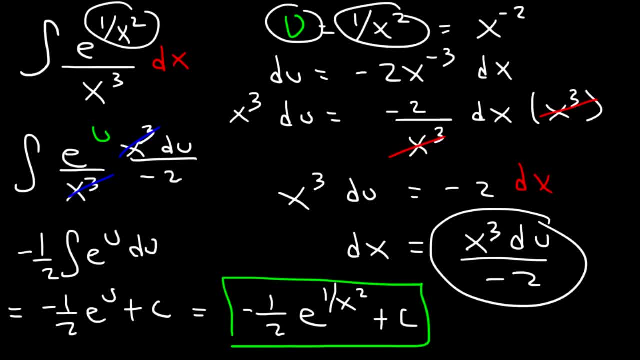 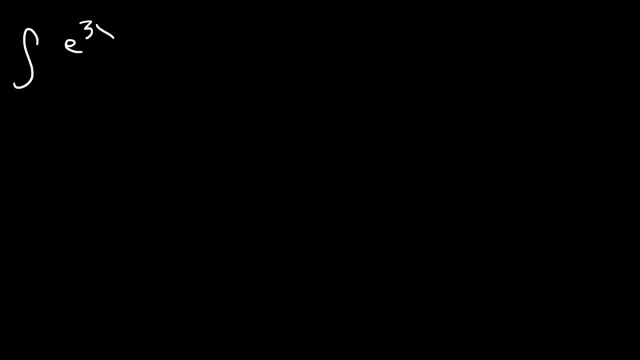 And that's it for this one. Now, what about this problem? What is the antiderivative of e to the 3x plus 4, e to the x plus 5, divided by e to the x dx? What do you think we should do here? 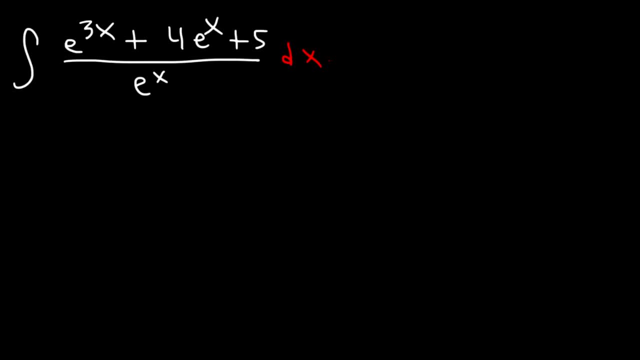 So we have a fraction and there's only one term in the denominator. What we can do is split the fraction into three smaller fractions, So it's e to the 3x over e to the x plus 4, e to the x over e to the x. 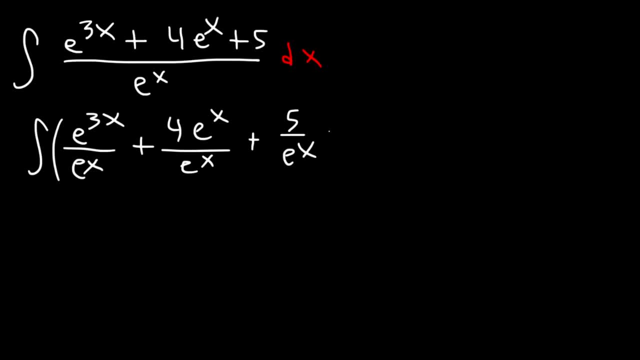 Plus 5 over e to the x. Now, what's e to the 3x divided by e to the x? Well, if we go back to algebra, x to the 7, divided by x, squared is x to the 5.. You need to subtract the exponents. 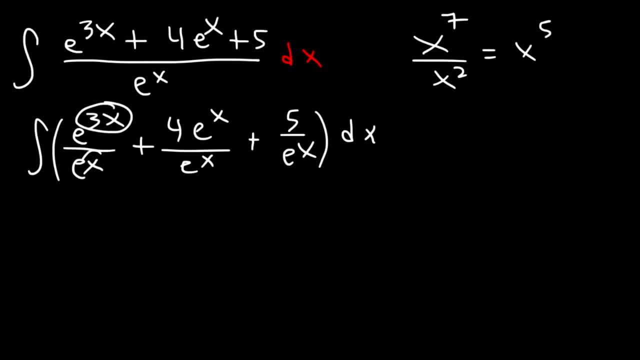 7 minus 2.. So here we've got to subtract the exponents: 3x minus x, or 3x minus 1x is 2x. So right now we have e to the 2x. Now for e to the x. 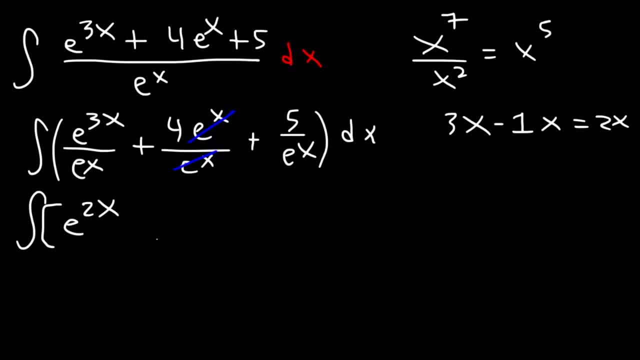 So for e to the x, these cancel because they're the same. x minus x is 0. So you just get 4.. e to the 0 is 1. by the way, Now this e to the x, we can move to the top and it will become e to the negative x, or. 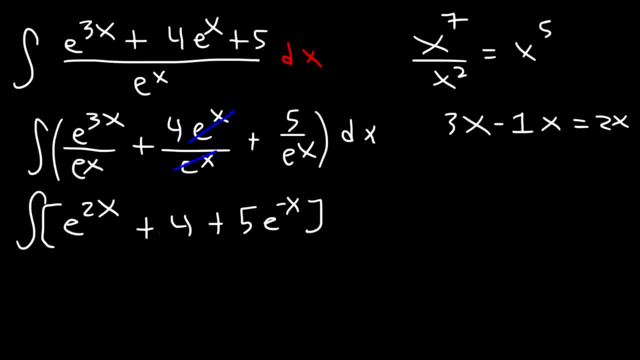 5. e to the negative x. And now we can integrate it in this form: The antiderivative of e to the 2x is simply e to the 2x over 2.. Integration of 4 is just 4x.